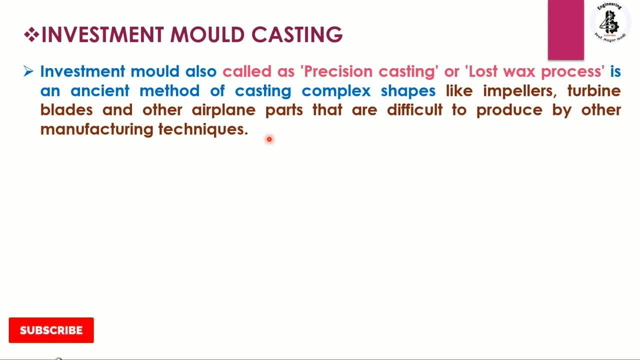 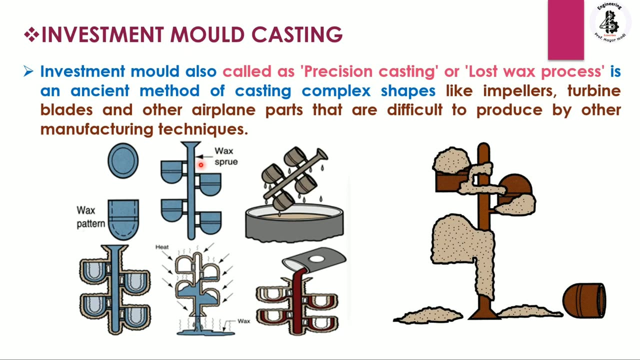 highly grade components with the help of investment mold casting process, which will be also used to making a high, precise and small size of the casted components. So basically, just you can see the various steps is being followed to making a investment mold casting process. So in this video we are discussing these all steps, along with the advantages and 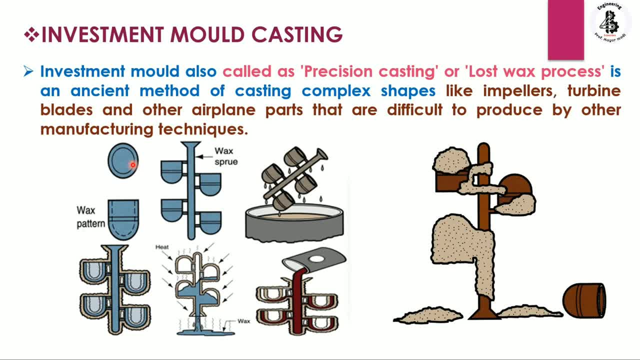 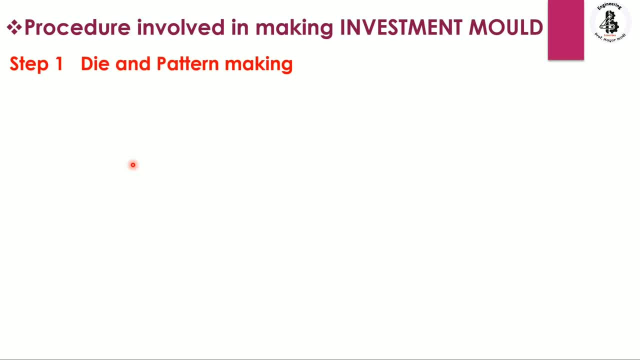 limitations of the investment mold casting process. So let us start with the first steps of investment mold casting process. So first of all, in step number one, dye and pattern making. So just you can see, this is our pattern making process. So basically the pattern materials here that will be a wax materials, So wax materials that will be easily 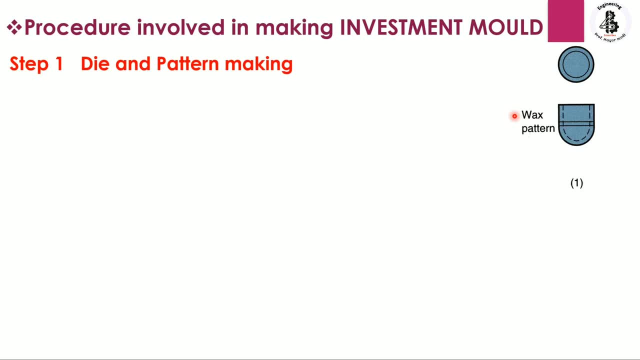 converting into desired shape and size as per my requirements. So in this process wax material- it will be used as a pattern materials. So a wax pattern is prepared by ejecting the liquid wax into a pre-fabricated dye having a same geometry of the cavity. 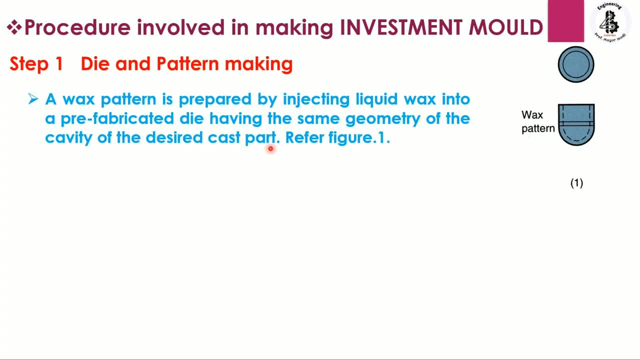 of the desired cast products. So, with the help of dye materials, this liquid form of the wax which will be introduced, and making the wax patterns as per my requirements, Then just you can see into the second steps that will be the sprue mechanisms. or you can say here: 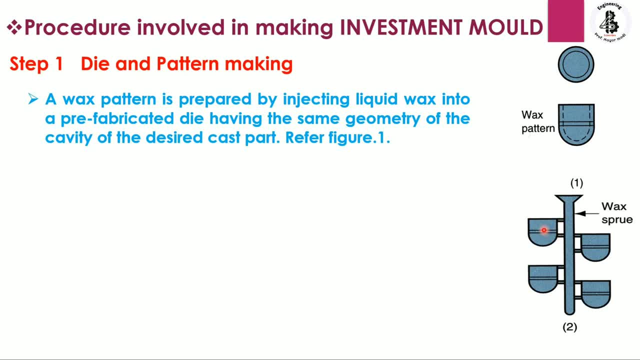 that will be making a one kind of patterns, or you can say jobs kind of shapes along the both the sides of the wax sprue. So just you can see the several such patterns are produced into the similar manners and then attached to a wax gate. 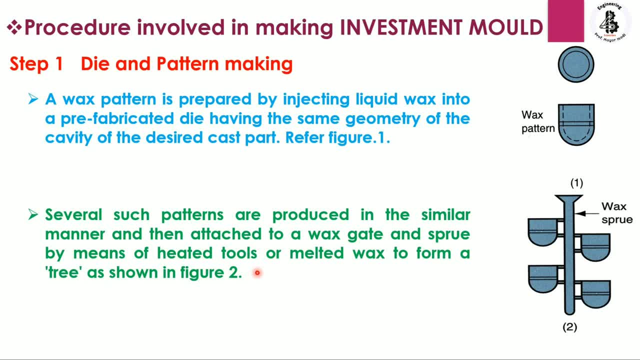 So in this process wax material will be used as a sprue, by means of a heated tools or melted wax to form a tree kind of shapes. So if there will be the requirement of the same size and shape of the components, so that will be attached from both the sides with the help of these kind of gating. 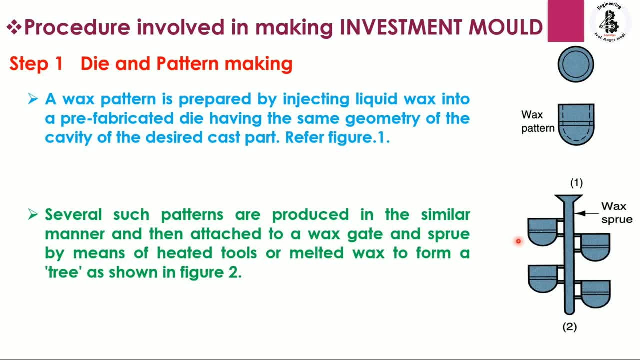 mechanisms. So in this process that will be the one of the advantages if you want to make the these similar kind of shape and size kind of components. So you just make a patterns as their shapes and it will be attached along both the side with a wax sprue, with a gating systems. Then after just you can see for the 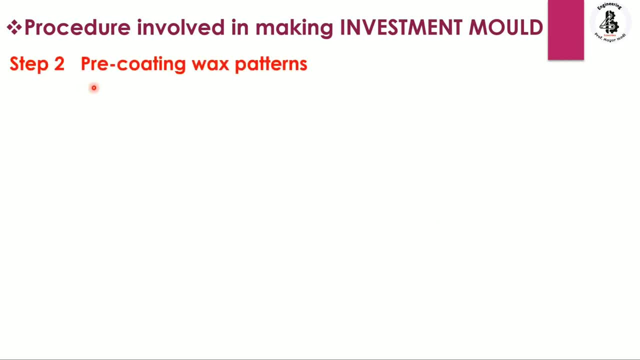 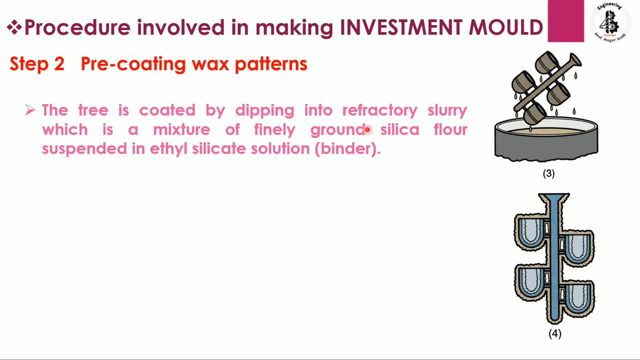 investment molding process. so in second step, pre-coating wax patterns. So just you can see. so these wax patterns, it will be poured into the coated environments. or you can say, this tree is coated by dipping into a refractory slurry. So basically this slurry that will be made with a mixture of the finely ground silica floor. 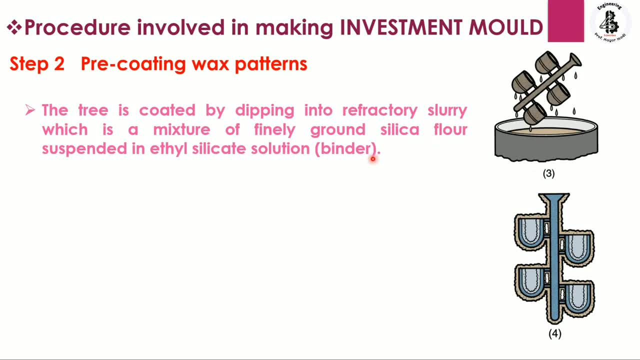 suspended into the ethyl silicate solutions. So this ethyl silicate solutions, it will be act as a binder. So just you can see these mixtures, it will be stick around this wax tree because this is a pattern materials and that will be wax materials. 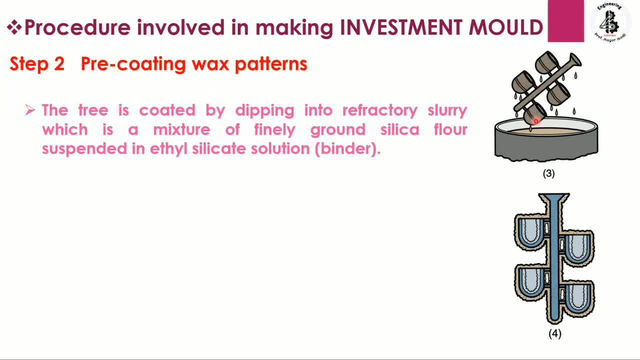 So that will be easily coated onto the wax pattern. Then the coated tree is spring with silica sand and allowed to dry. So that is our figure three and four. So after dipping the this wax tree, now the this mixtures, it will be stick onto the outer side. 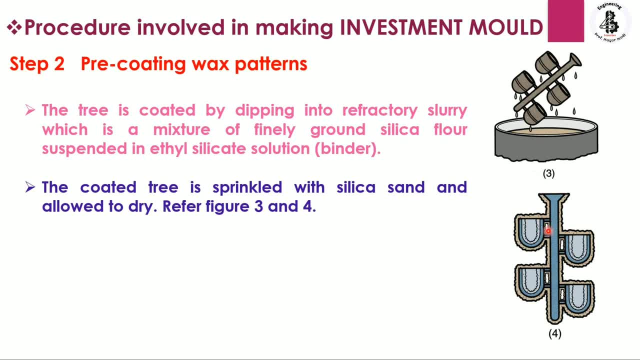 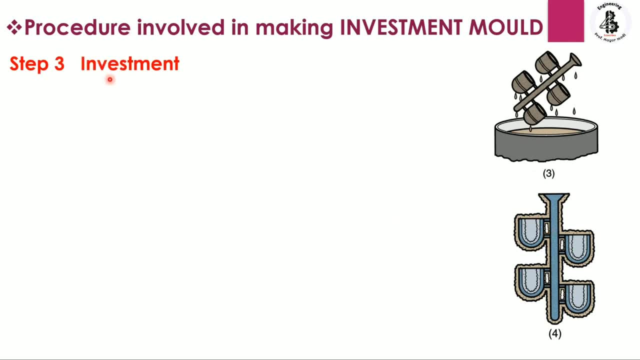 and it will be make it dry. So after this, what happens? just you can see that will be the step number three, So that will be investment. So what is the meaning of that? the pre-coated tree is coated against, So that will be one kind of investment. So by dipping in a more viscous slurry. 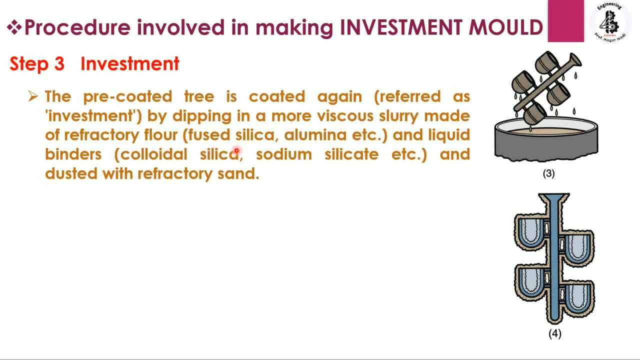 and made a refractory floors. So basically fused silica alumina that will be used, and liquid binders as a colloidal silica, sodium silicates as a binder and dusted with a refractory sand. So that will be the investment. So the process of the dipping and dustings is repeated. 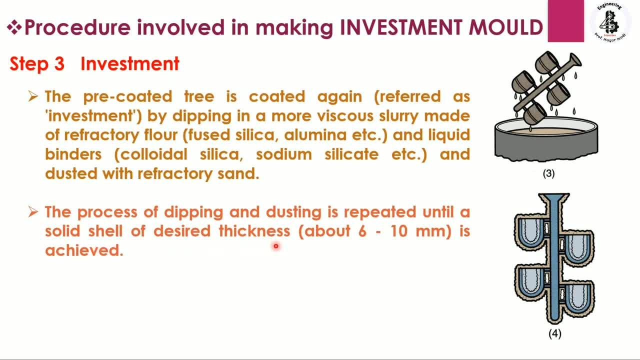 until a solid cell of the desired thickness- So generally that will be around six to ten mm- is being achieved around these wax patterns. So, as you can see, this mixer of the slurry with the binders that will be sticking onto that particular outer side of the wax patterns. 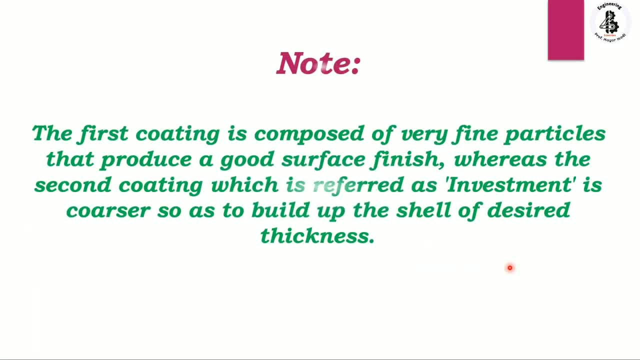 Then the some important notes for the investment molding process. the first coating is composed by very fine particles that produce an antimossless, likedeath good surface finish, whereas the second coating, which is referred as a investment, is coarser, so as to build up the 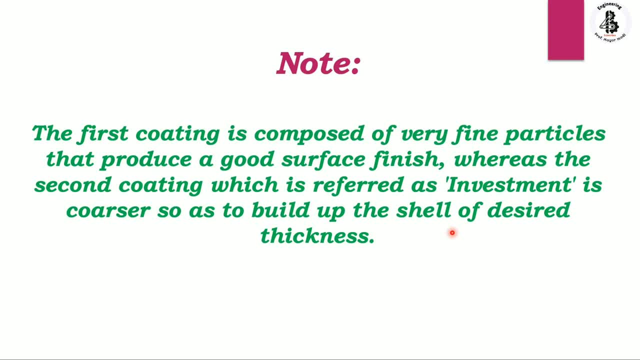 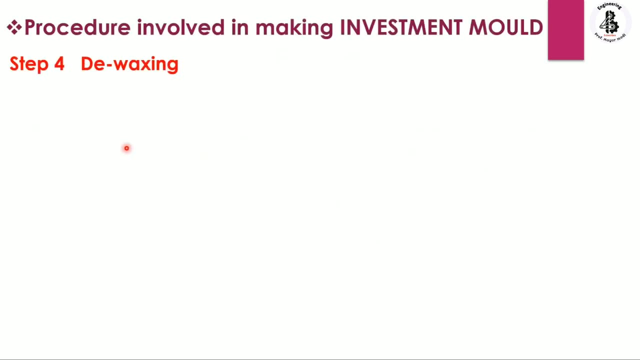 shell of the desired thickness. so basically, that second dipping that will be increasing the strength or you can say thickness of that particularly slurry components. then into the investment mode, the next steps that will be de-waxing. so just you can see, by the heating of that particular all 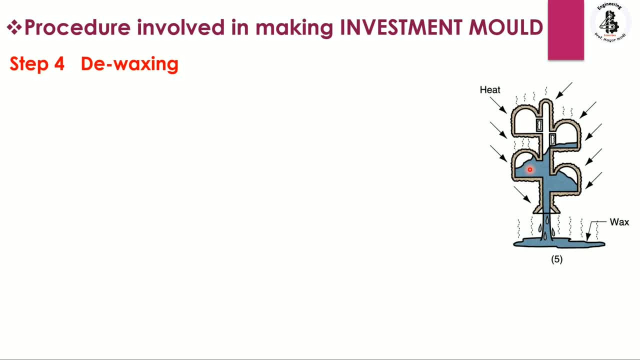 the components. so what happens? these wax materials? it will be in the form of the liquid, so that will be easily run away from these patterns, right? so it will be making the one, this kind of cavity, right? so just you can see, in these steps the tree is placed in an inverted positions and heated. 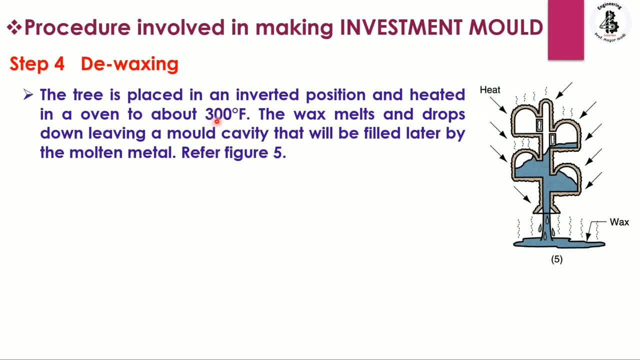 in an oven to about 300 fahrenheit. so the wax melts and drops down, leaving a mold cavity that will be filled later by the molten form of the metals. so this is the way it will be inverting and heated. after this, the reheating, the 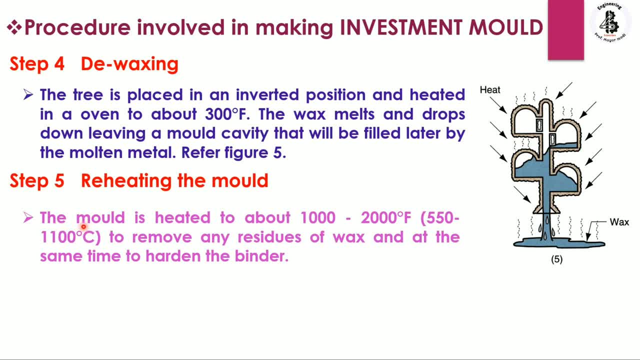 mold, mold. so basically the mold is heated about 1000 to 2000 degree fahrenheit, or you can say around 550 to double one, double zero degree centigrade to remove any residuals of the wax, at the same time to harden the binders. so that will be also increasing the 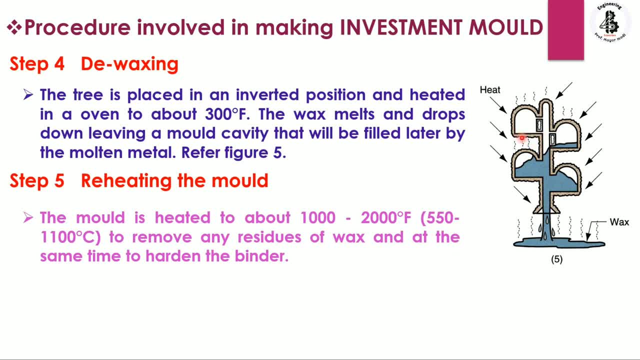 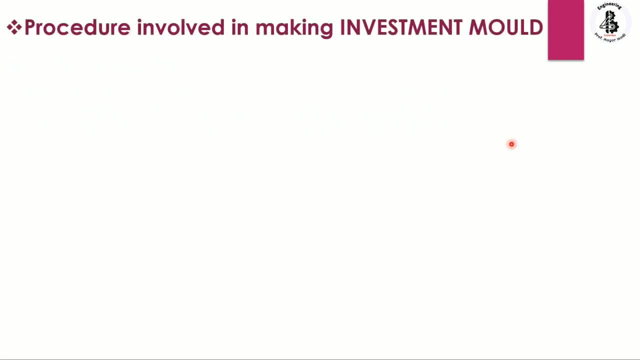 strength of that, particularly mold cavity which will be made with the help of wax tree, or you can see, the mold cavity will be made as a mold cavity, or you can say wax materials, then after, in step number six, melting and pouring, just you can see once again it will be inverted and just 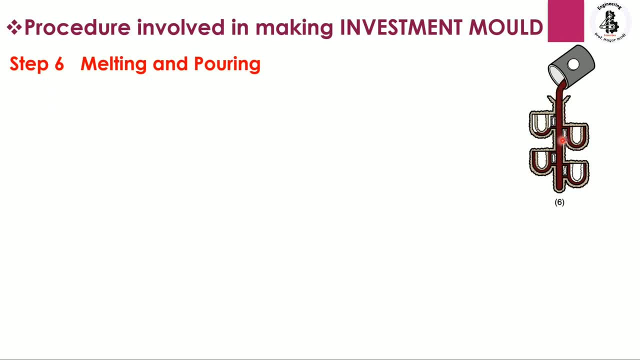 you can see the molten form of the metals which will be pouring so by these two kind of mechanisms, and this one is our getting systems. so it will be poured into the mold cavity. so this one shape, or you can say cavity, that will be my required shape and size. 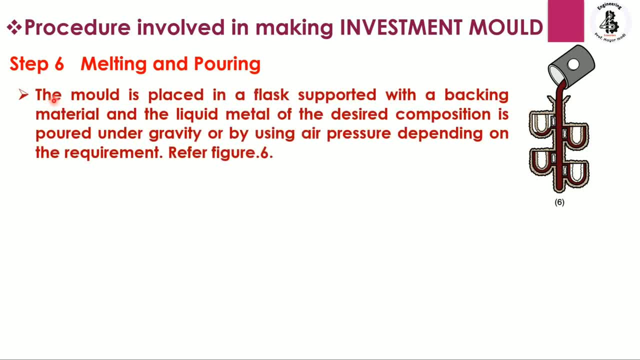 of my components. so the mold is placed in a flask supported with a backing materials and the liquid metals of the desired compositions is poured under the gravity or by using a air pressures, depending upon the requirements. if it will be the complex geometry, so you can use the 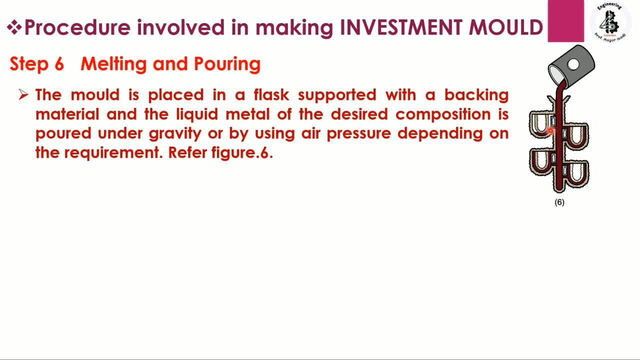 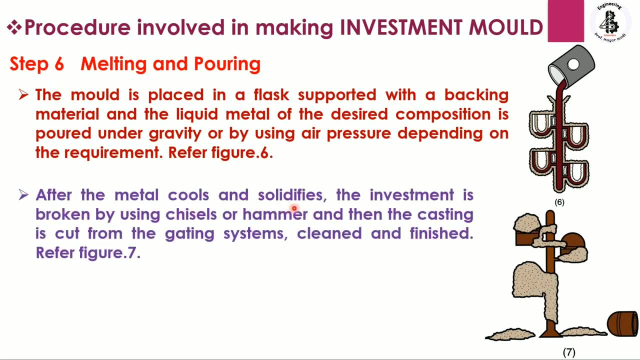 air pressures, otherwise it will be directly pouring into the mold cavity. then, final, after the metal cools and solidifies, the investment is broken by using chisels or hammer and then castings is cut from a getting systems and finish just. you can see these all sand particles, or you can see. 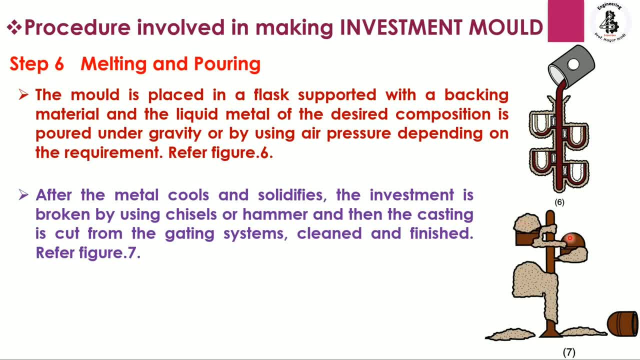 investments that need to be removed. so this one we are doing on this, so this one we are doing on this and this one we are doing on this and this one we are doing on this. just you can see, these all are the required shape and size of the metallic. 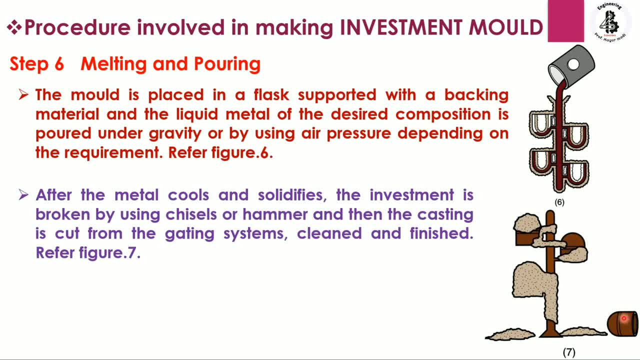 materials. so this one is our final shape and size. so this is the method of the investment mold casting process, or you can say investment is being used to making the components. the major advantages of this process is what that will be used for: making a small size of high precise components in the single 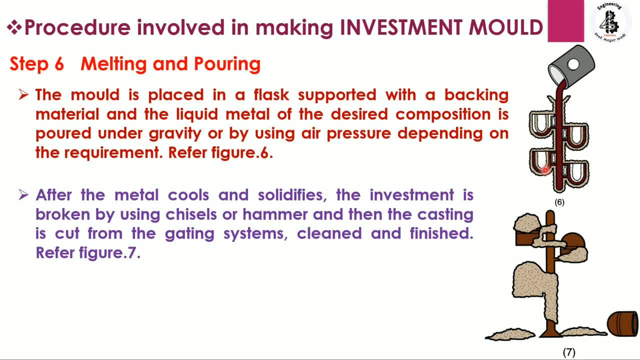 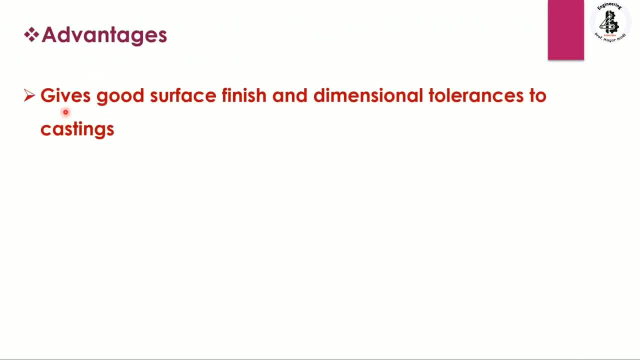 wax tree. you can also make the different shape and size of the components. and some of the advantages: gives good surface finish and dimensional tolerance to the castings. eliminates the machining of the cost parts because it will be having a higher finishing at the end of the this process.